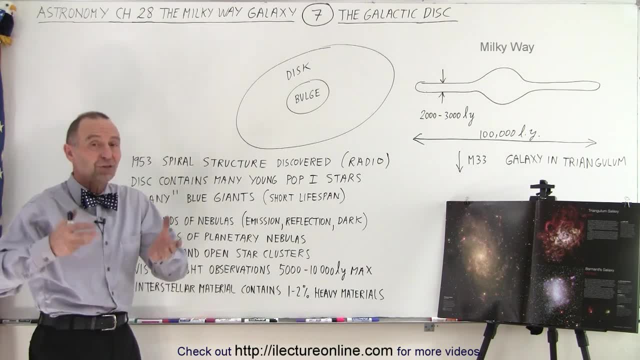 Now we then discovered that the Milky Way galaxy had a spiral structure, like we had discovered already for almost 200 years. to the telescopes, We saw these objects that we thought were spiral nebulas. Now we realize that, hey, they're actually galaxies. 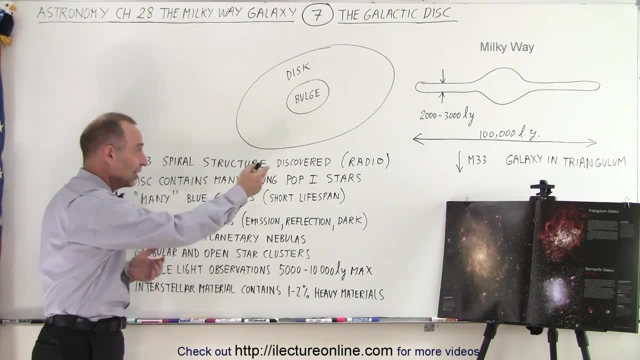 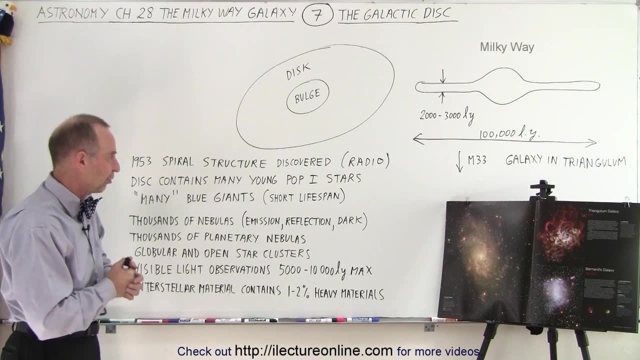 Not only that we now realize, since the onset of radio astronomy, we realize that our own galaxy had was of a spiral structure as well was a spiral galaxy. So the disk contains a lot of young, what we call young population, one stars. 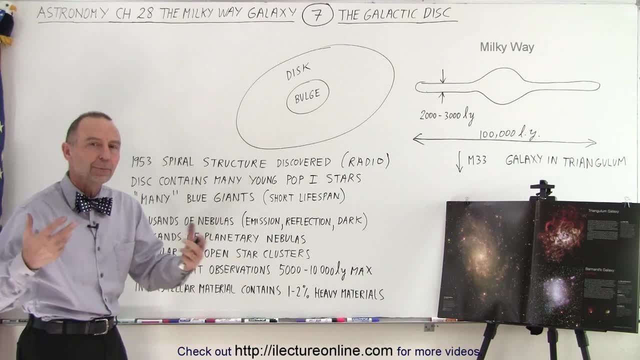 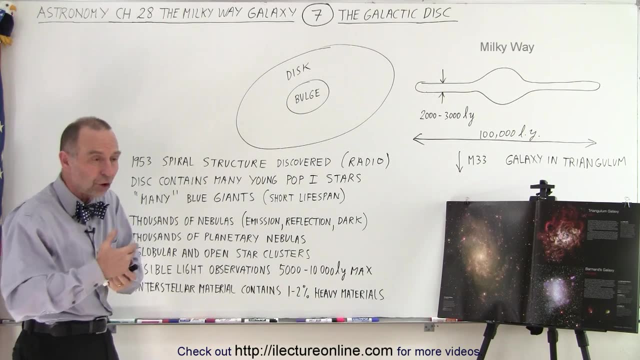 population one stars: the stars that are recently formed and that are formed out of the material that's been swirling around and that's been fed by the depth of these supermassive stars through these supernova explosions with the heavy materials, And so the younger the stars are. 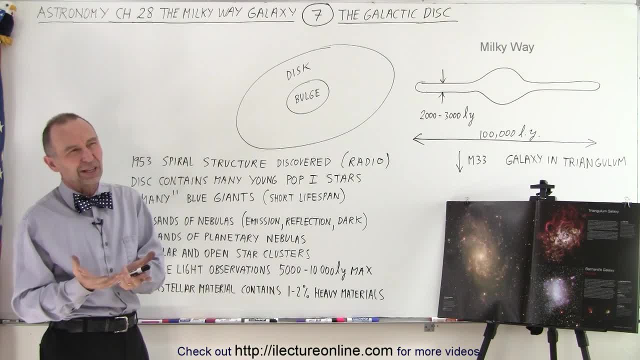 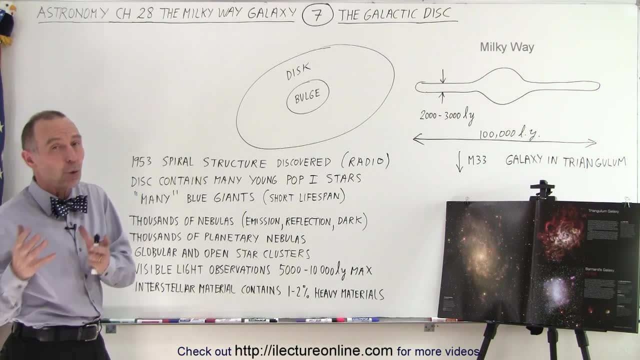 the more likely they will contain a lot of the heavy material. Now, when we say a lot, we talk about one to perhaps even 2%, which is enormous when it comes to a star, because most of the older stars are 99.9 or even more. 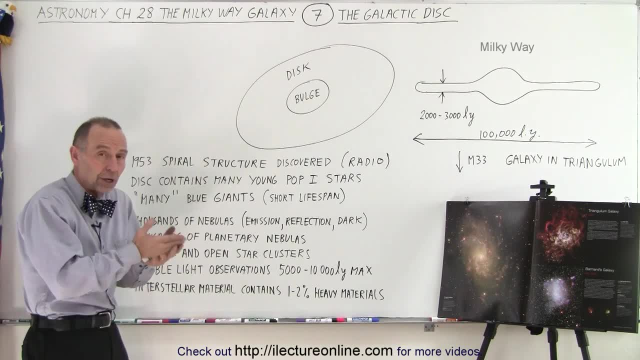 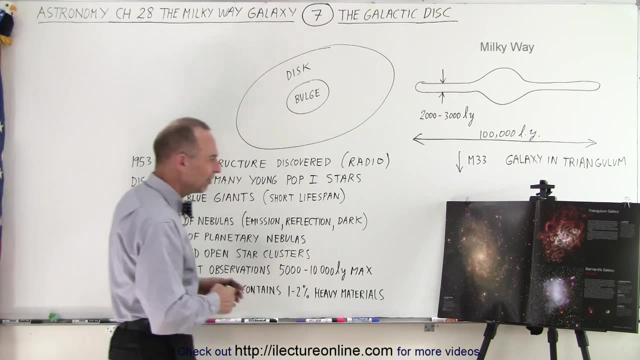 than 99.9% hydrogen and helium, where the newer population one stars can be as much as one to 2% of the other heavy materials. We also see a lot of blue stars Now here in this particular picture. because of the coloration, you can't see the blue. 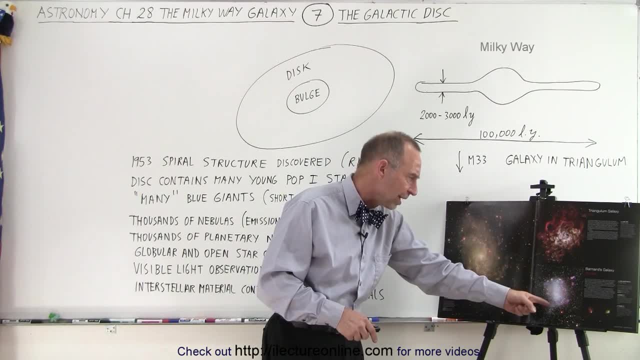 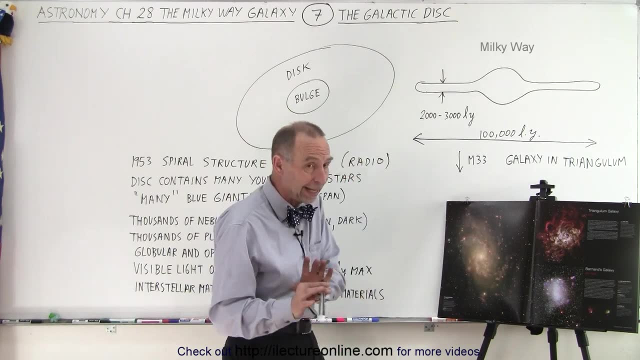 Here is one of those irregular galaxies. It's called Barnard's Galaxy and you can see the bluish color which typically you see in the spiral galaxies as well, as well as in M33, and as well as in our own Milky Way galaxy. 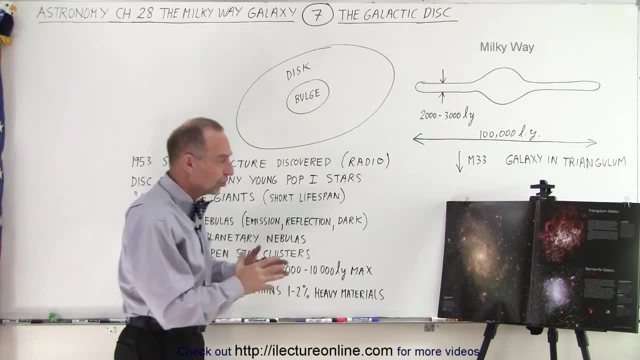 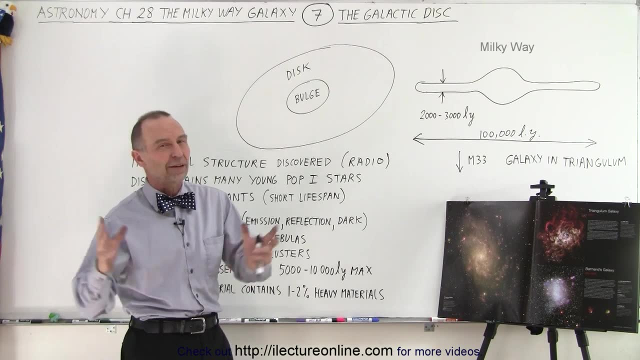 So you can see that in the disk region, not only do you see a lot of nebulas, you also see a lot of bluish color from these enormous blue giants that are being formed Now. blue giants have a very short lifespan. 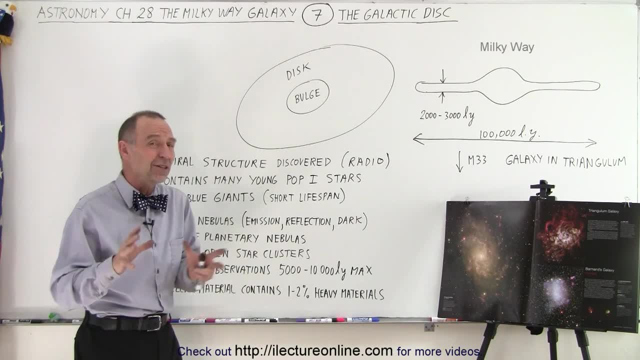 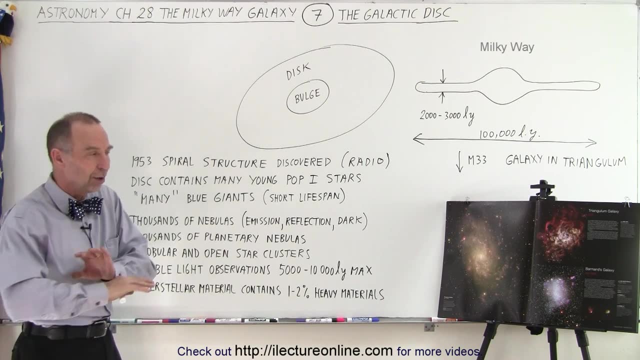 anywhere from 10 to 50 million years- 100 million years max- before they turn into red giants. So when you see a lot of blue stars, you realize you're looking at a lot of very young stars. Blue simply means there's a lot of new stars being formed. 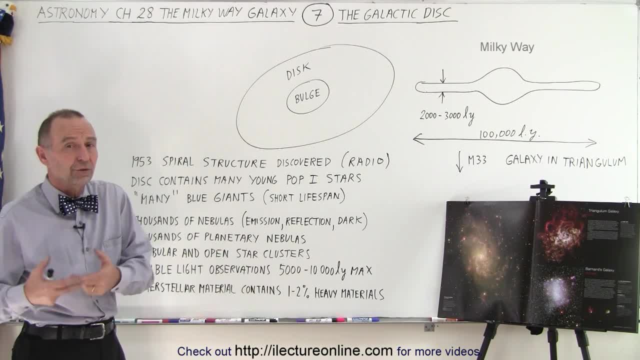 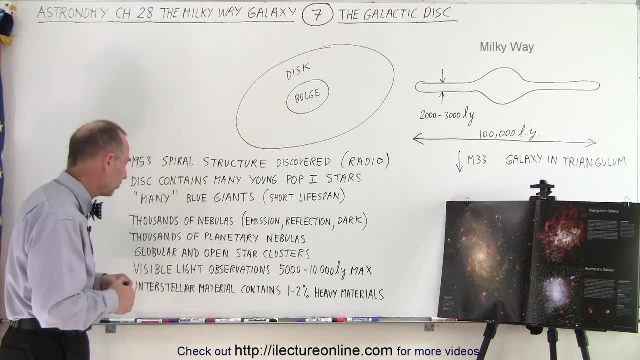 because typically only one out of a thousand or one out of 10,000 stars being formed are actually blue giants, And so if you see a lot of blue giants, there's a lot of formation of a lot of stars taking place. So the thousands of nebulas include the emission nebulas. 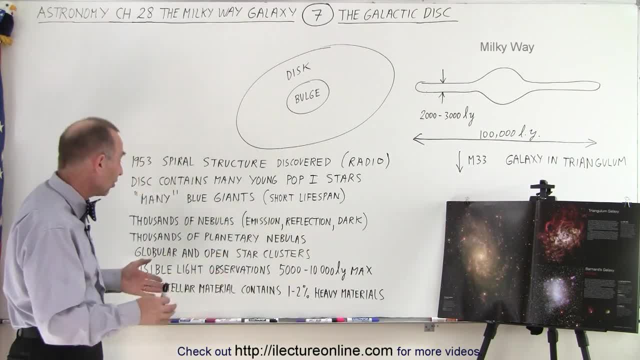 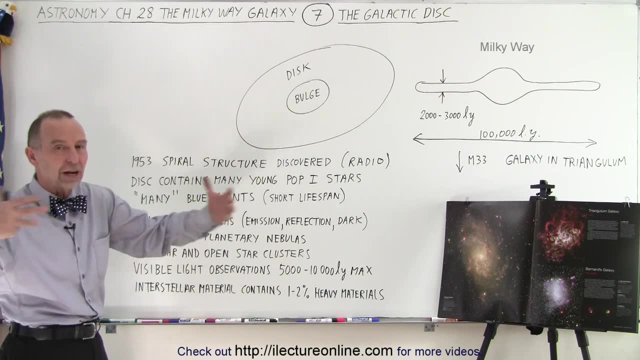 reflection nebulas, dark nebulas, you name it, they're there. In addition to that, of course, there's thousands of planetary nebulas, because those are the end result of normal size stars that then shut off their outer layers. 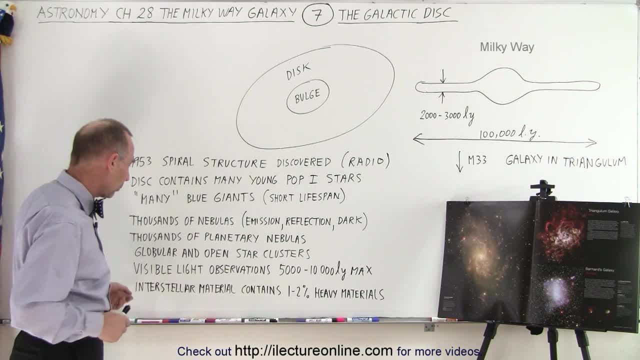 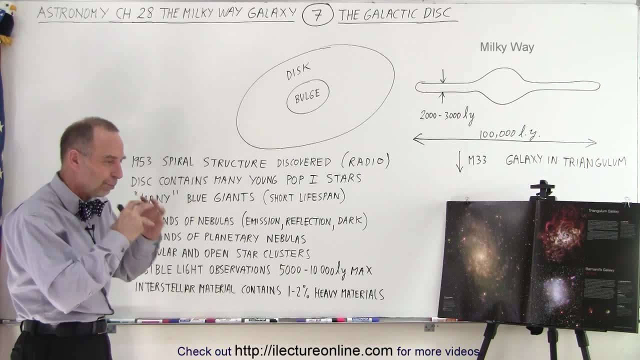 which then for a while, become planetary nebulas. We also have a lot of globular and open star clusters, Globular or globular, however you want to pronounce it. So these are just big star groupings. The globular star clusters are enormous groupings of stars. 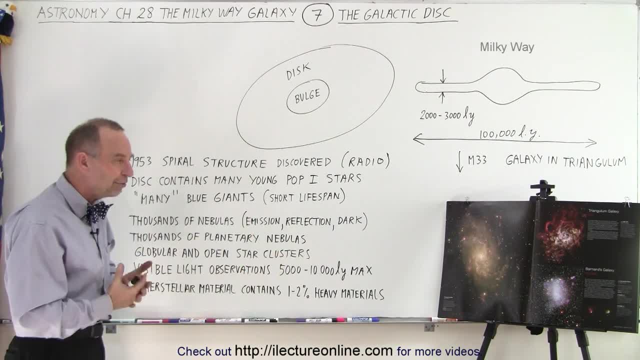 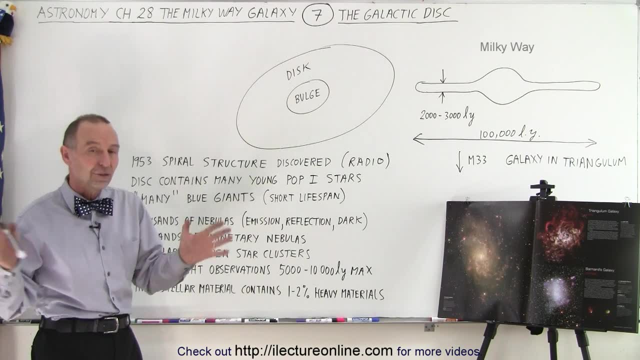 The open star clusters are a little bit further spread out. There's more of them, but there's not as many stars in each of the open clusters, But all throughout the disk. you can see the globular clusters and some of the globular clusters. 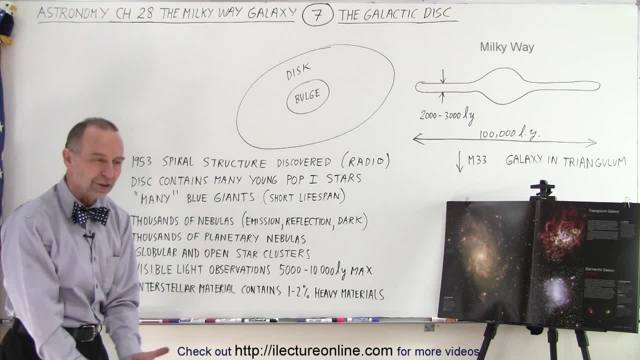 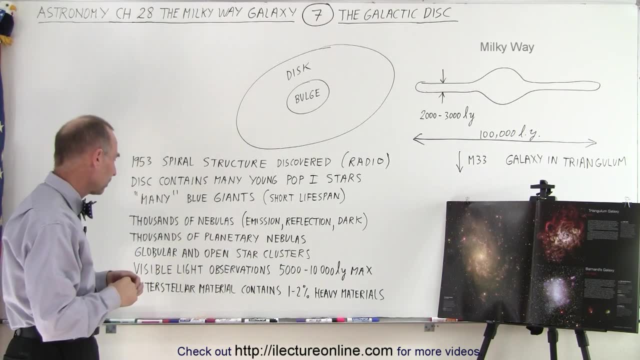 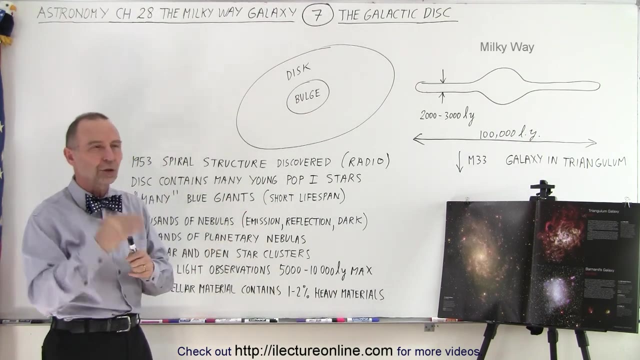 Remember, the globular clusters are kind of like a bee swarm in a spherical region around the galaxy, including the disk and the bulge. So yes, even in the disk we find some globular clusters. Visible light observations are limited because of all the dust and all the nebulas inside the disk. You can only see so far in the disk before you start, before the light gets blocked by all these hindrances. So we can typically only see about 5,000 or 10,000 light years into any direction, especially when we start looking towards the center of our galaxy. 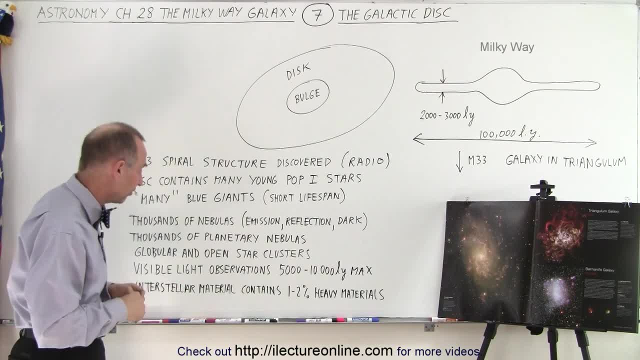 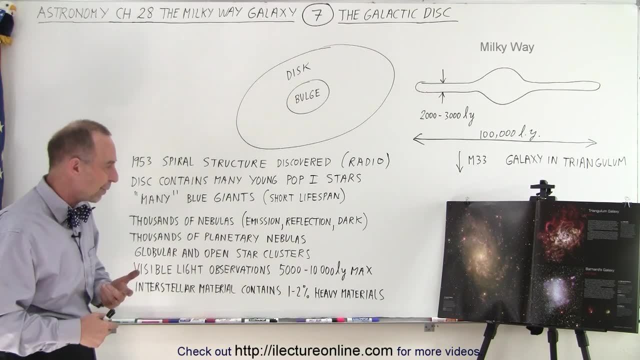 There's not a lot to be seen there, because the light simply gets blocked, So visible light observations tend to be limited to about 5,000 or 10,000 light years. Beyond that we need to start using infrared radio X-rays. 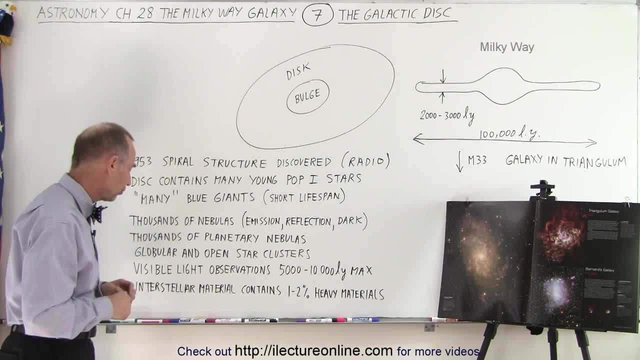 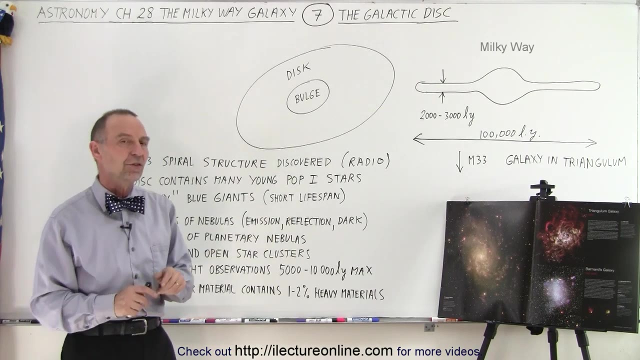 other forms of radiation to be able to see, to peer through some of those very heavy, dense regions of gas and dust. And then the industry, the interstellar material itself, so the material that's spread out between the stars, between the nebulas that fill up all the remaining material between the stars. 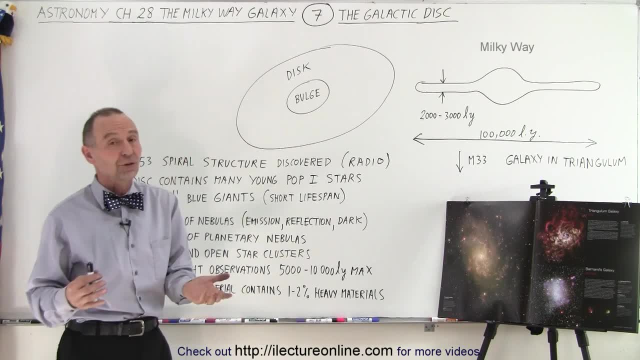 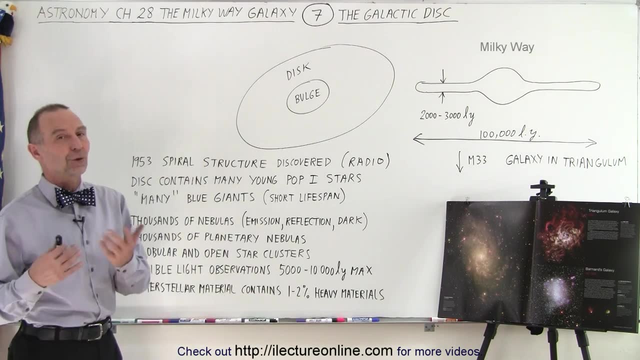 well, it turns out that about 1 to 2% of that is heavy materials. So any new population of stars being formed will contain a lot of the new heavy materials, And those are then potentially places where planetary- not planetary, but terrestrial- planets can be formed. 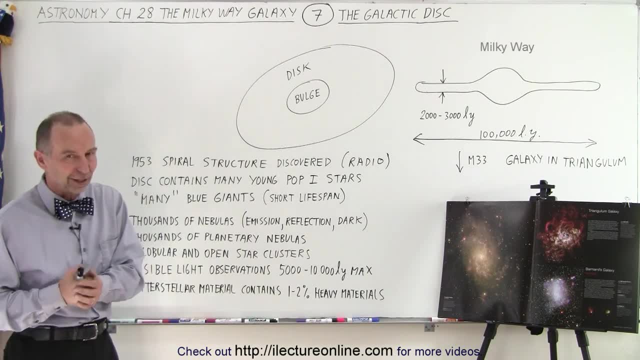 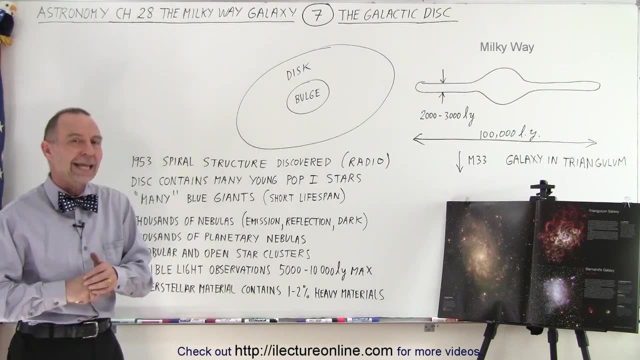 because you need the heavy materials to form planets like the Earth. So that's why newer stars are the places you want to look for Earth-like planets, not the old population two stars. They probably don't contain any terrestrial planets, probably just the gas planets.